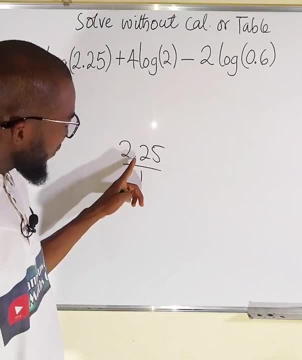 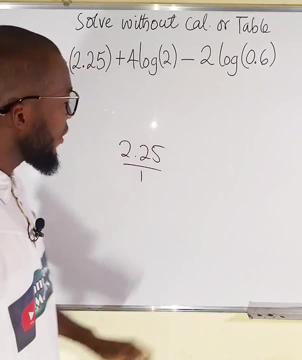 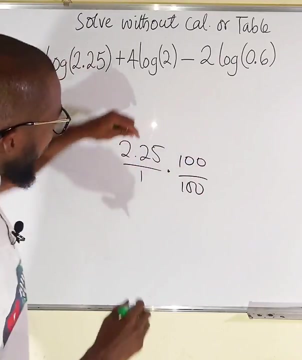 2.25 divided by 1. and this point, if I want to migrate it to the last significant number, I have to multiply by 100.. So for equivalent fraction, we can multiply the top and the bottom by 100, so that this becomes 2.25.. 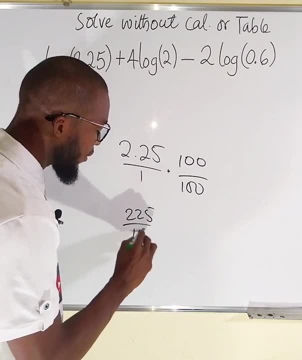 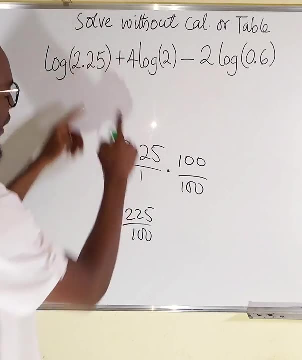 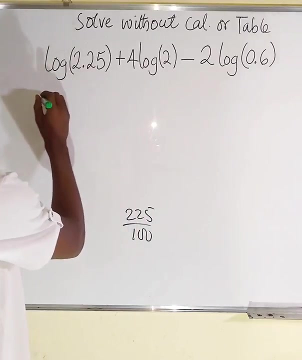 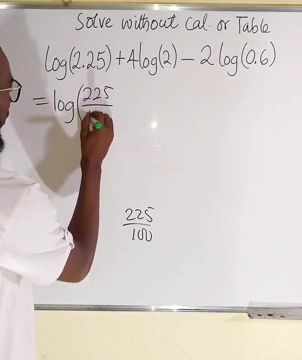 5 and 1 multiplied by 100 is 100. This is only because I want to show you all the details. So instead of 2.25, I can now write it as 225 divided by 100. So we have log of 225 divided by 100.. Next let us move on to the second term here. 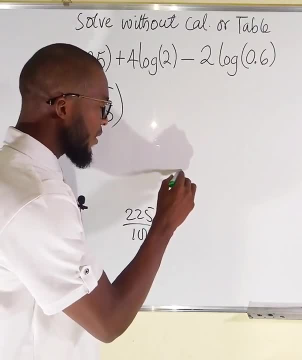 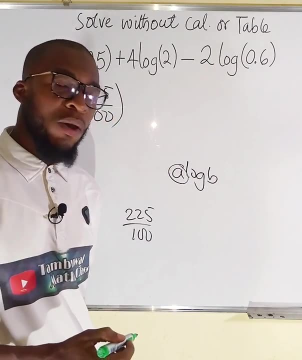 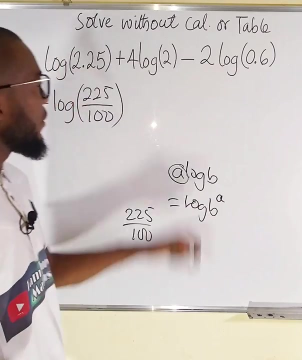 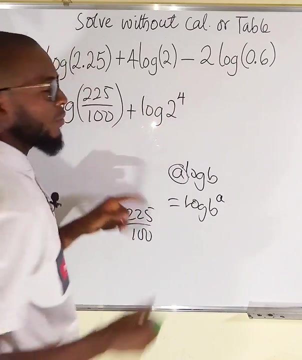 Remember, we have a law of logarithms that says: if you have something like a log b, this a right here can always serve as the power of b. so instead of this, we can write it as log of b, power e. so we can write this as log of 2, power 4.. Again, we can apply the same thing here, minus. 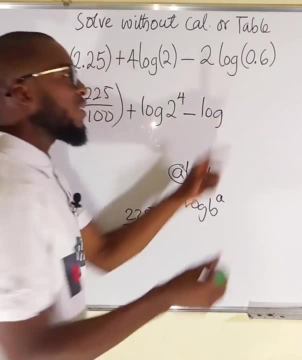 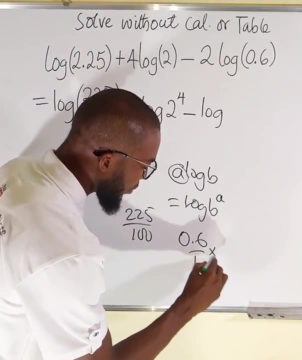 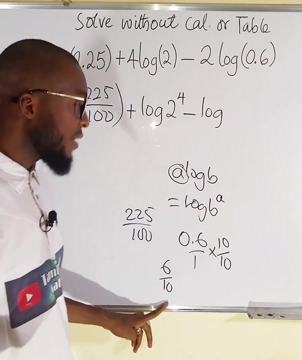 log of oh. 0.6 can be written as 0.6 divided by 1. we can multiply top and the bottom by 10, so that this becomes only 6 divided by 10.. Therefore, 6 divided by 10 is the same thing as 0.6. 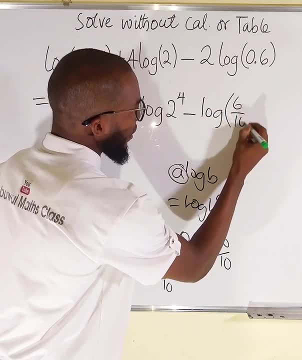 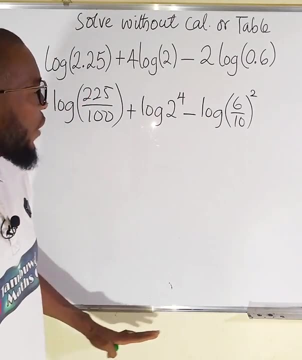 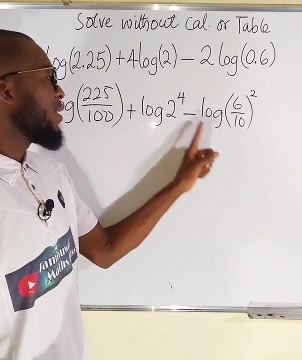 so we write 6 divided by 10, all to the power of these two right here. Moving on Now we are going to apply one law that says: if you have addition, you can multiply and give them a single log. If you have subtraction, you divide and give them a single log. So we can now assign. 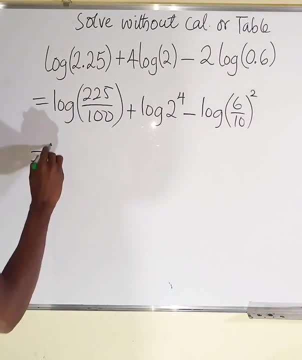 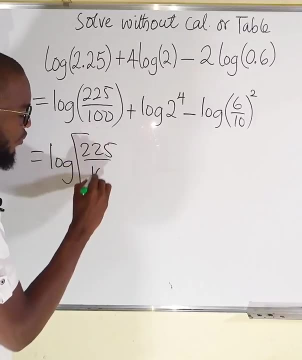 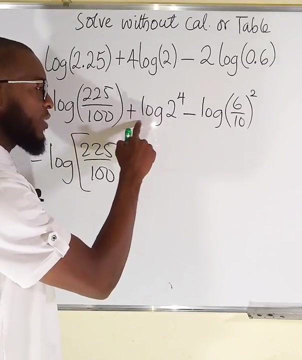 them all with a single log. So we have log of all. what we have here is 225 divided by 100.. Remember that 2 power 4 is 16.. So instead of addition, we multiply by 16 and I can rationalize it as 16 divided by 1.. 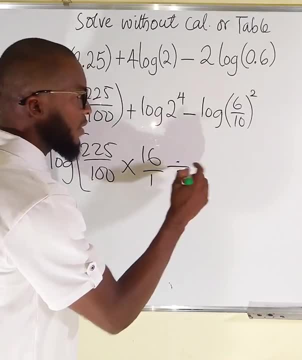 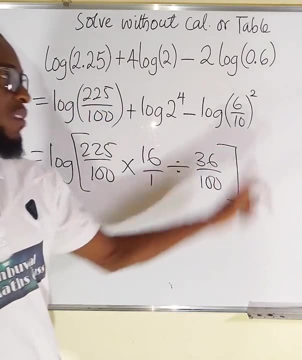 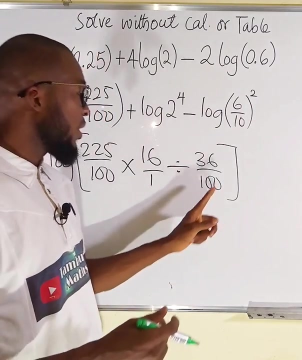 Then instead of subtraction we have division sign. then this is: remember, 36 divided by 100, because 6 power 2 is 36, 10 power 2 is 100. But instead of this division we can change it to multiplication and take the reciprocal of this fraction. 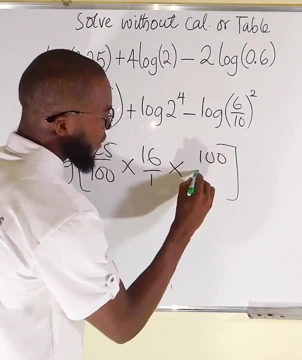 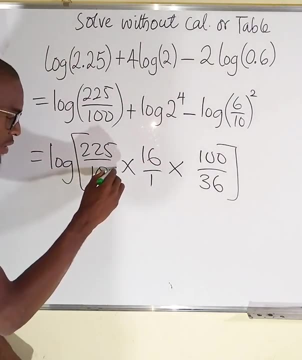 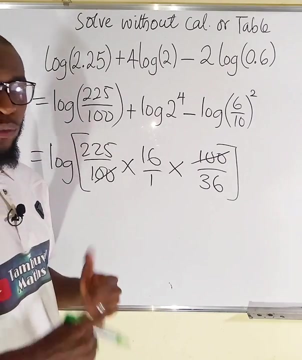 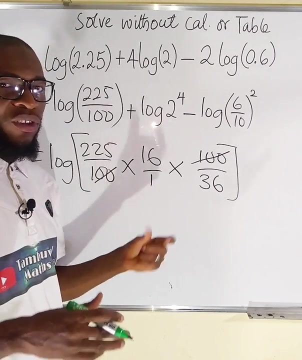 And instead of 36 over 100, we have 100 divided by 36.. From here we have all multiplications. 100 can cancel this 100.. What we have entirely under this bracket is 100. Why? Because 225 multiplied by 16 is nothing but 3600 or 3600, and if you divide it by 36, you shall obtain 100.. 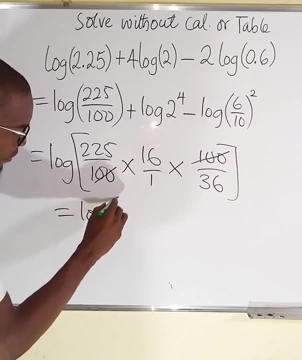 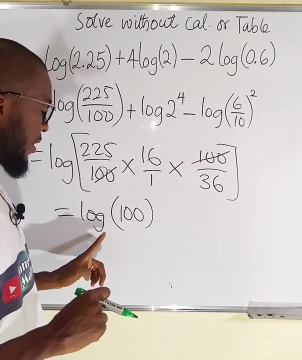 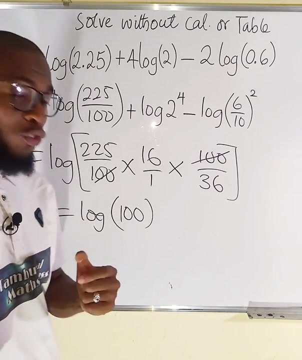 So this is equal to log of 100.. And remember that if you are dealing with a log without an assigned base, that log is in base 10.. Take note of that. This 100 can be written as 10 power 2.. So this is the same thing as log of. 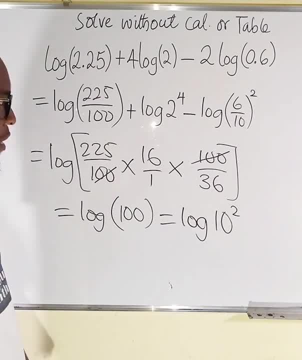 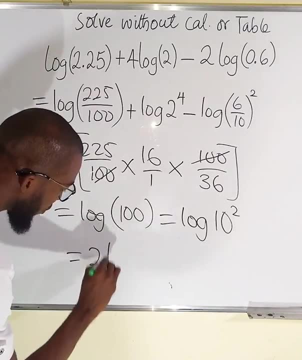 10 power 2.. 10 times 10 is 100. Then we can apply that law that says this power can now drop down to multiply. So this is equal to 2 log of 10.. Remember the base is 10.. 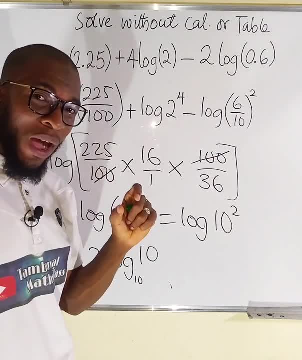 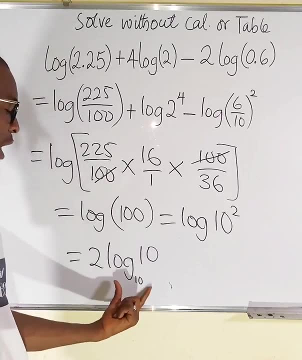 Another law that says log of a number having the same base as that number is equal to 1.. Therefore, log 10 base 10 is equal to 1 and 1 multiplied by 2 is equal to 2.. Finally, our answer is equal to 2.. 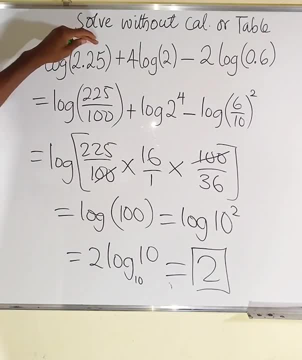 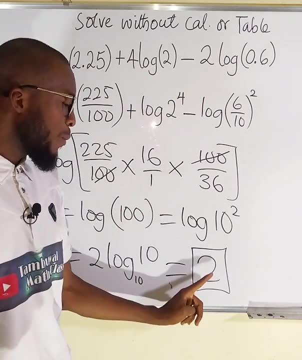 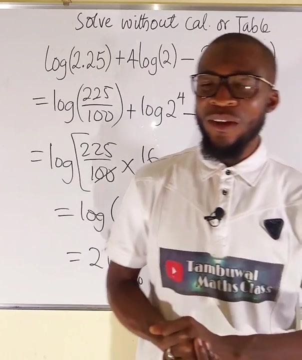 The whole of this expression here: Log of 2.253 plus 4, multiplied by log of 2 minus 2, multiplied by log of 0.6, is nothing but equal to 2, and this is all I have for you today. thank you for watching. do share to your learning colleagues and don't. 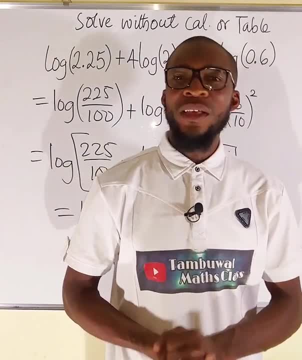 forget to subscribe to my youtube channel for more exciting videos. bye.